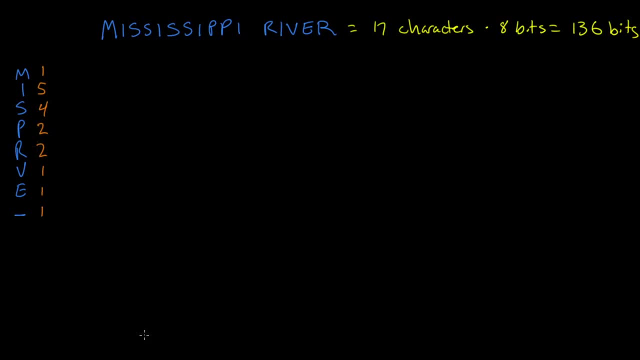 forth Next. sort these by their frequency of occurrence. I'm going to sort them with the greatest number on the left-hand side and the least number on the right-hand side, In order. that would be I5, S4, P2, R2, M1, V1, E1, S2, and so on. 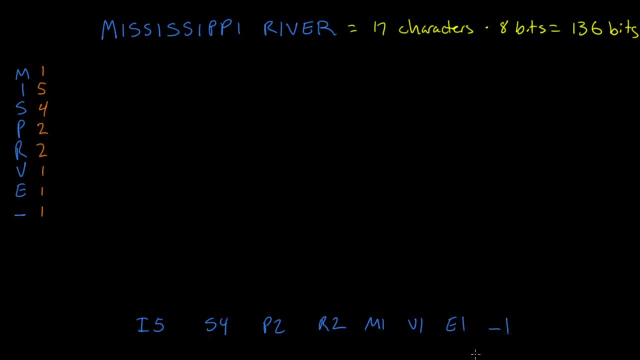 We're going to be building a tree out of this by merging together nodes and combining them into one. Start by looking for the two nodes with the lowest numbers. We've got four to choose from here, so it doesn't really matter which ones we look at. Let's 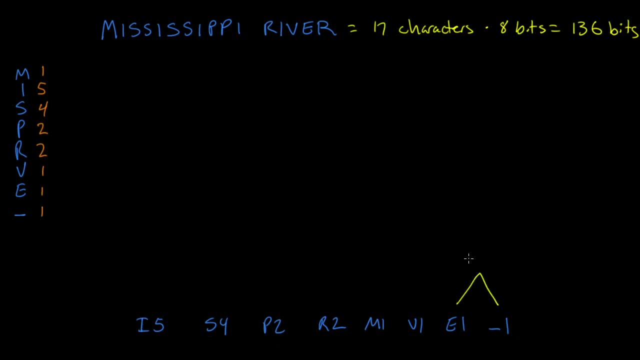 do E and space. We're going to combine those together and those become E, space with a sum of 2, because 1 plus 1 is 2.. Repeat, Find the two nodes with the lowest numbers and merge them together: M and V. M and V combine to make a sum of 2.. And repeat again. Now we're going to find 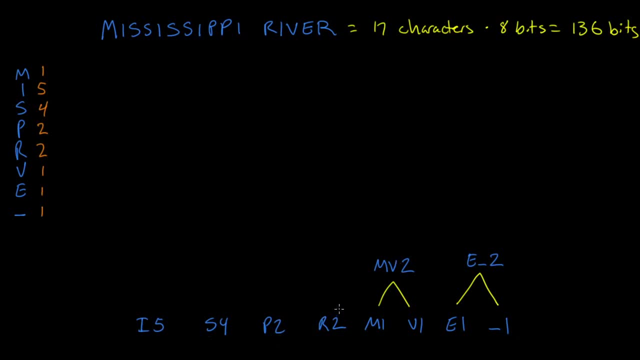 the two with the lowest numbers. There's four to choose from. It doesn't really matter which ones we choose. Let's do P and R. We'll merge those together and make P R 4.. And we just keep repeating: We've got 2,, 2,, 4,, 4, and 5.. Let's do the 2 and 2.. This becomes M V. 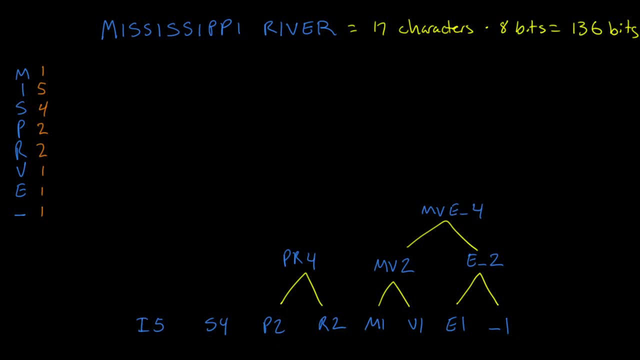 E space 4.. Repeat again: Let's do P? R merged with M? V E space, And this is going to become P? R M V E space, with a total of 8.. Now we've got 5,, 4, and 8. We need to choose the two with the lowest numbers, so we'll. 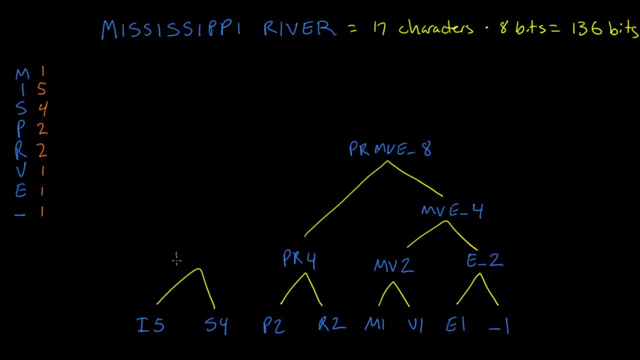 choose 5 and 4, and we'll merge those together. I S 9.. Now we've got 9 and 8. Merge those together. I S P R M V E space with a total of 17.. A good double check is to make. 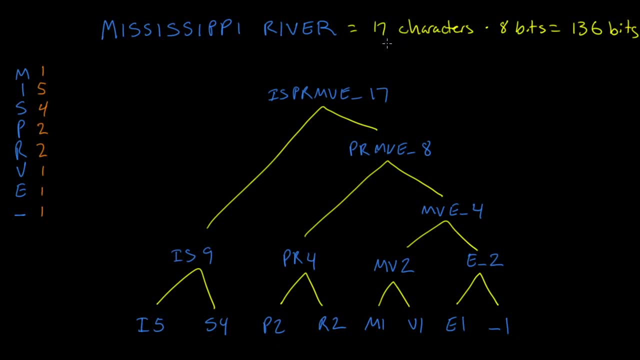 sure this number here, 17 at the very top, is equal to the total number of characters in our original and also equals the sum of all these numbers here on the left-hand side. The last thing we're going to do to the tree to complete the construction is to label the. 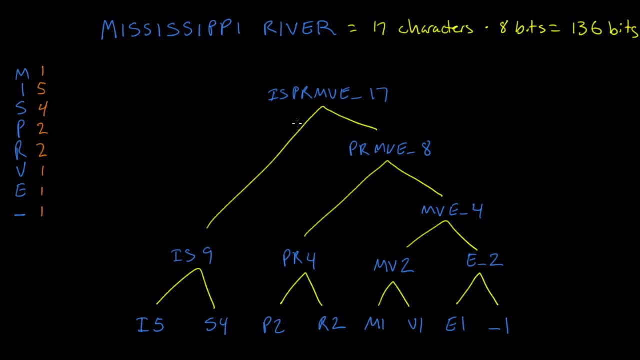 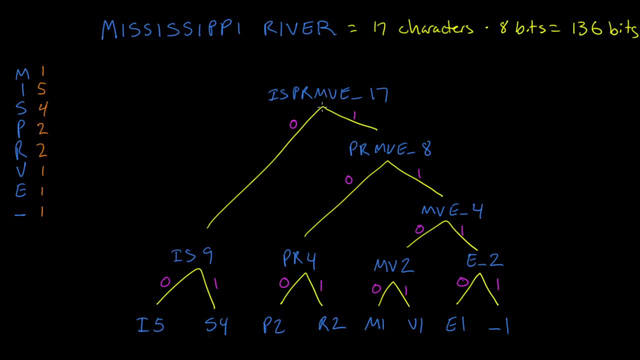 To find the binary encodings for each one of the letters, just start at the top of the tree and follow each one of the branches down to the letters. Here's the encoding for I: We start at the top branch, follow the 0 down and then follow the next 0 down. So the encoding. 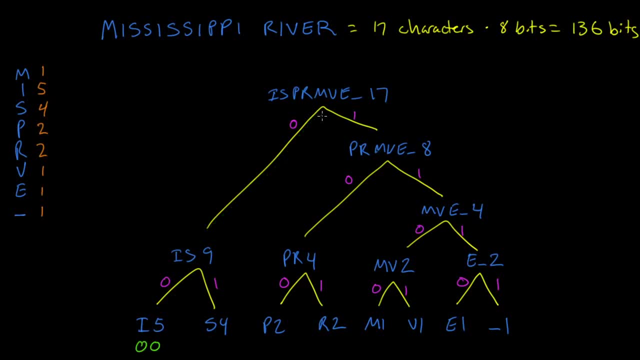 for I is 0, 0.. To find S, start at the top, follow this, branch down and then follow this one down. This one is then 0.. 0, 1.. P is found by going to the right and then to the left and to the left. Its encoding. 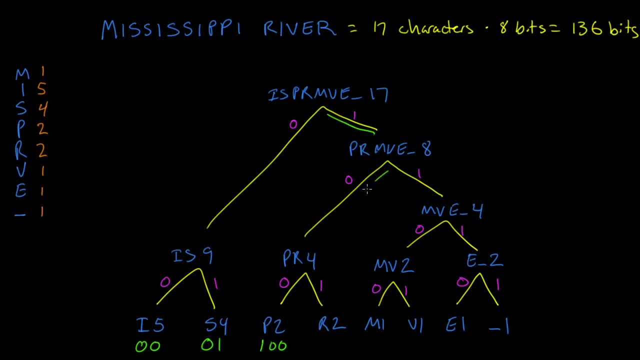 is 1, 0, 0.. Do the same thing for each of the other letters. Now look here: The letters with the greatest frequency have the shortest bit representations and the letters with the lowest frequency have the longest bit representations. So we're. 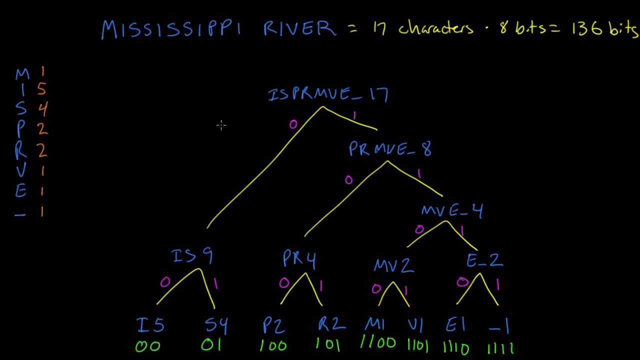 done with the bit representations. That's exactly what we wanted. We don't need this tree anymore. All we need are the letters and the bit representations. Now we can write out the bits for our message. Start with M. M is 1, 1, 0, 0.. I is 0, 0. S. 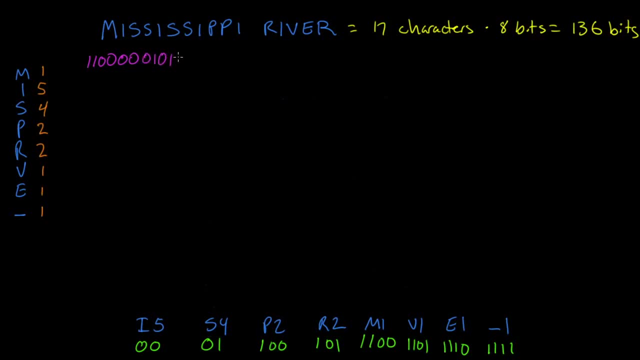 is 0, 1.. S is 0, 1, again I is 0, 0.. 0, 1 for S, 0, 1 for S: 0, 0 for I. P is 1, 0,. 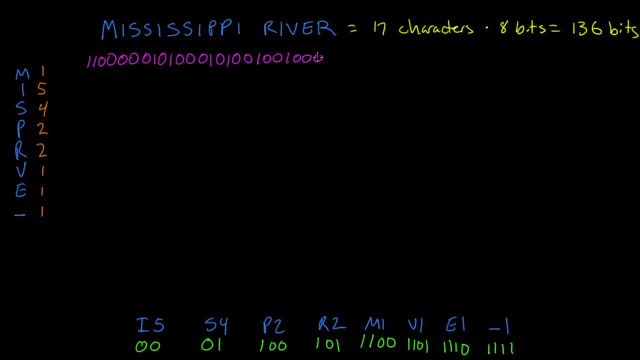 0.. 1, 0, 0, again 0, 0 for the I Space is 1, 1, 1, 1.. Keep doing this for the rest of the message. And there's our Huffman-coded binary message for Mississippi River, If I've. 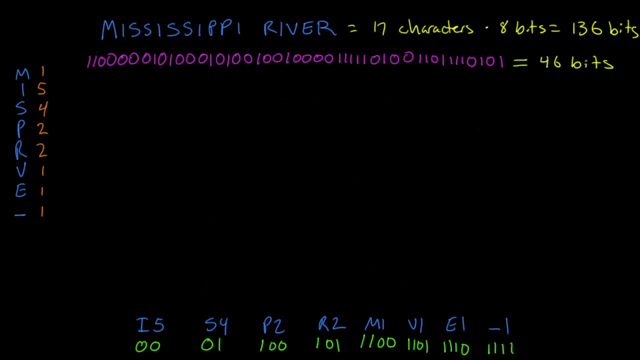 counted these upright, there are 46 bits in this message. That's a dramatic savings over the original 136 bits needed for the message. In fact, 46 bits is about 33% of the original one. That's a savings of close to 67% over the original message.